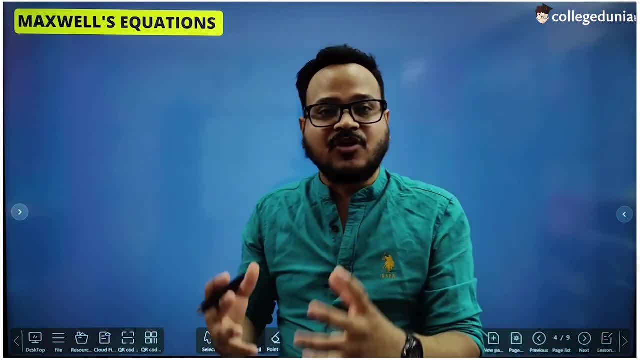 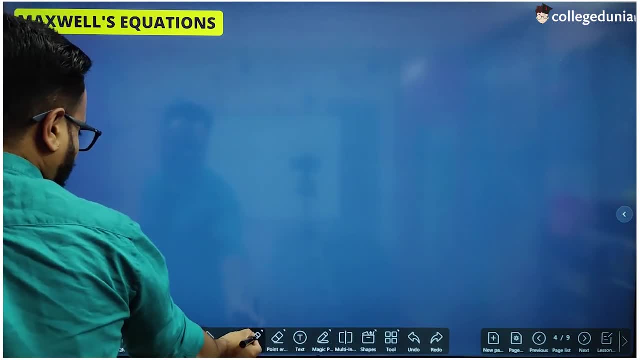 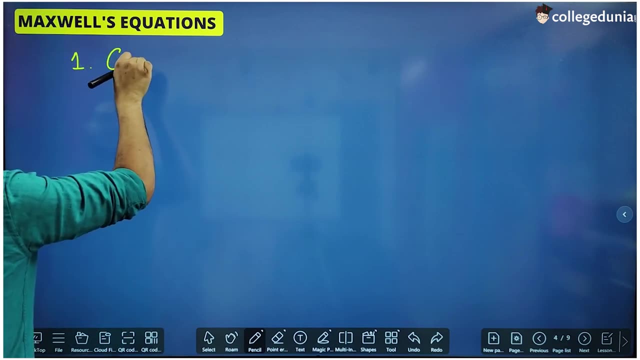 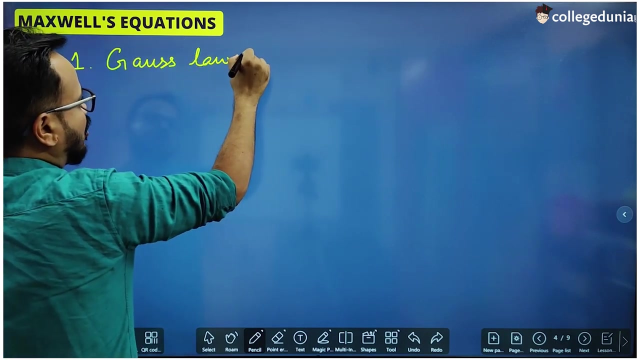 as Maxwell's equations. All the concepts, all the fundas of electromagnetism are covered in those four equations only. So what are those equations? Number one, from electrostatics. Maxwell picked Gauss law in electrostatics and this is the first Maxwell equation, Gauss law in. 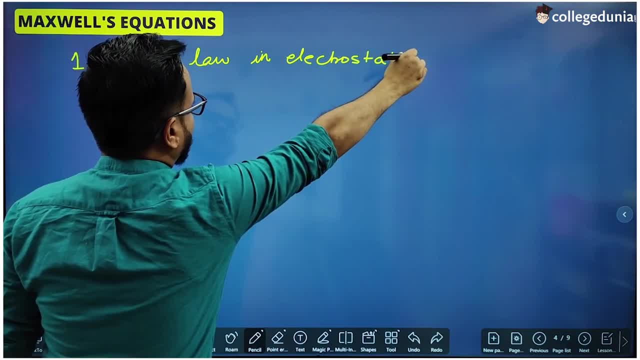 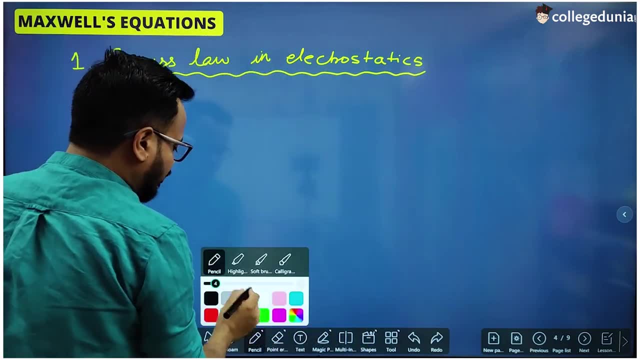 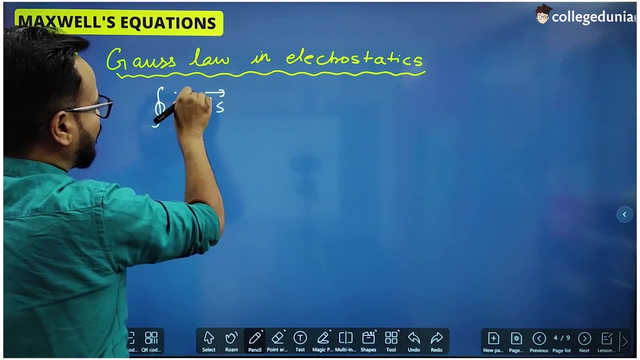 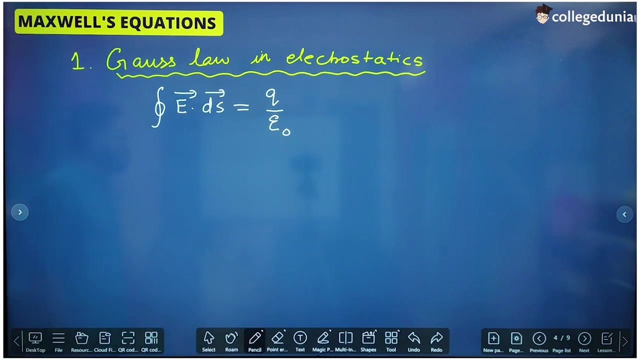 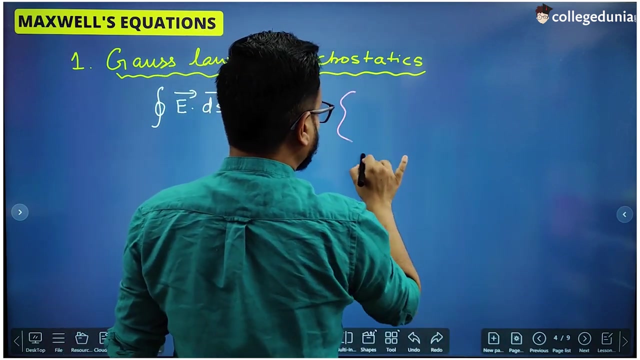 electrostatics. What is Gauss law? We all know that Gauss law is that the surface integral of electrostatic field, that is, the total electric flux through a closed area, is 1 upon epsilon, naught times the total charge inside that surface. For example, this is a closed surface and this closed surface contains a charge Q, then the total. 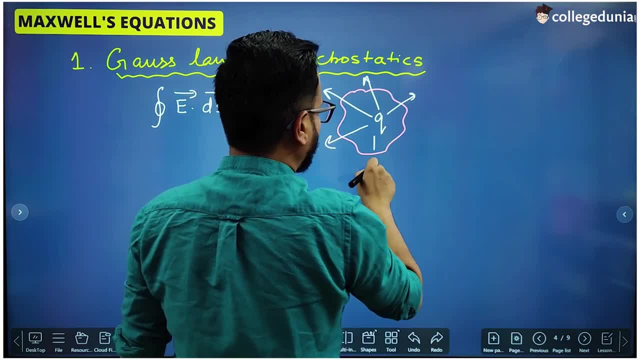 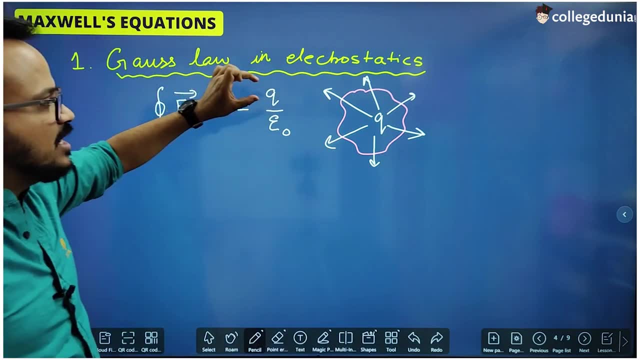 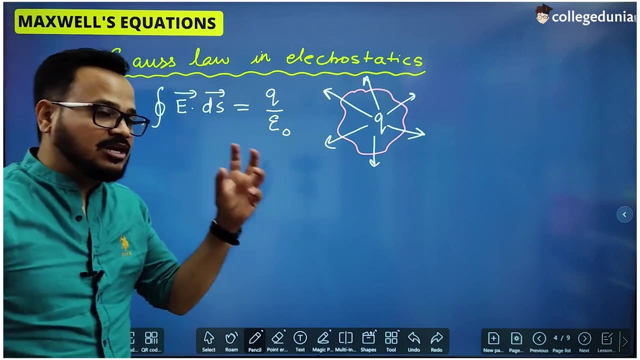 electric flux, that is the total number of electric field lines which are coming out of the surface. If you want to calculate the total flux through this surface, you will just divide this Q by the value of epsilon naught. If you want to see this in detail, you can. you can refer to the lecture of. 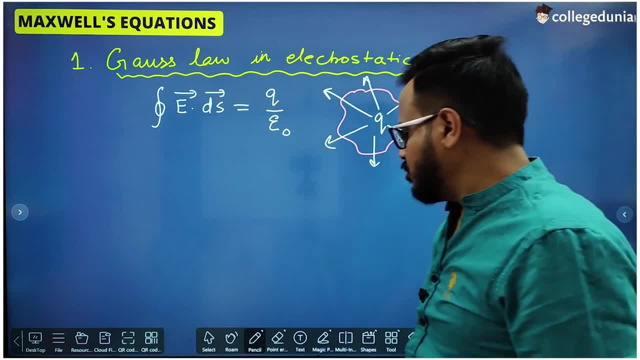 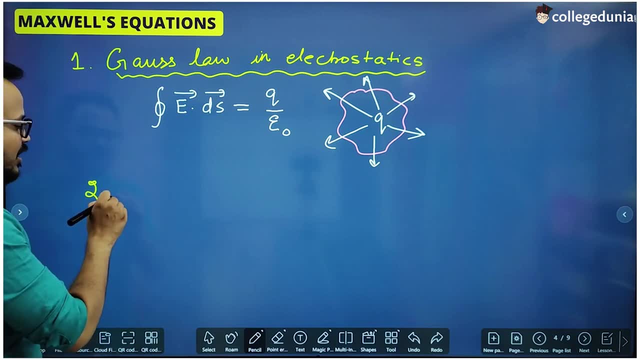 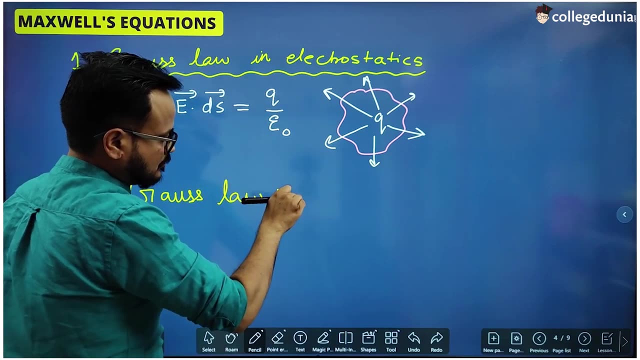 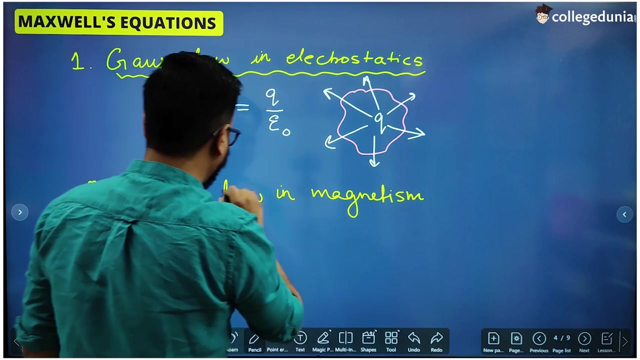 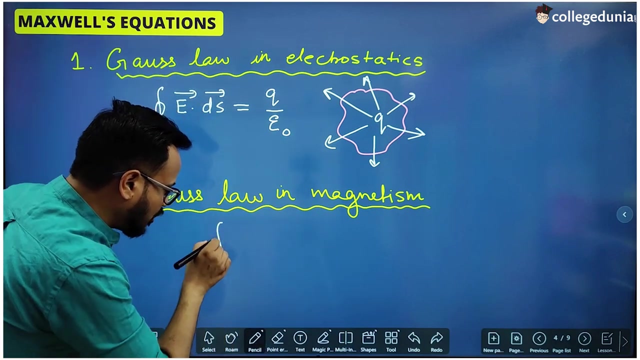 Gauss law on this channel. Now we have seen in what was the first Maxwell equation From magnetism. Maxwell picked again the Gauss law in magnetism and this is going to be the second Maxwell equation. Gauss law in magnetism simply says that the total magnetic flux 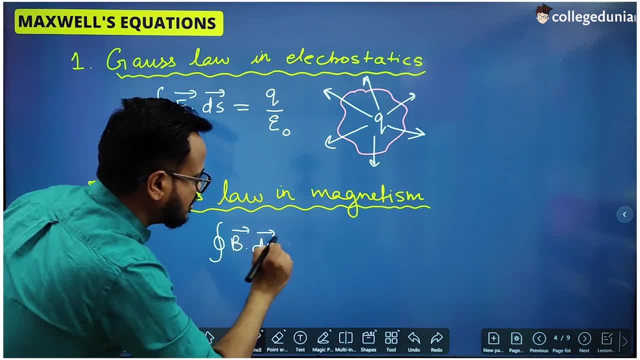 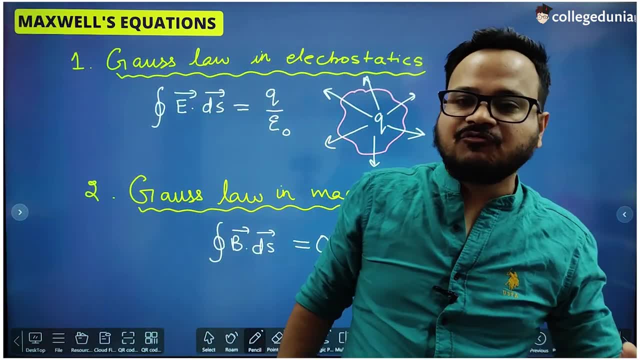 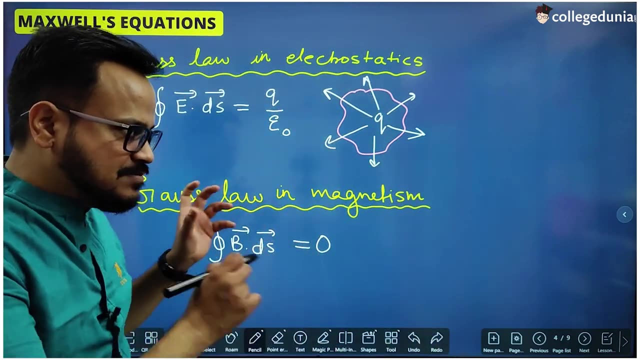 that is, b dot ds through a closed surface is always zero, because if there is a source of magnetic field inside a closed surface, then that source must have both north pole and south pole of the same strength, because you cannot separate north and south poles from each other. north and south both. 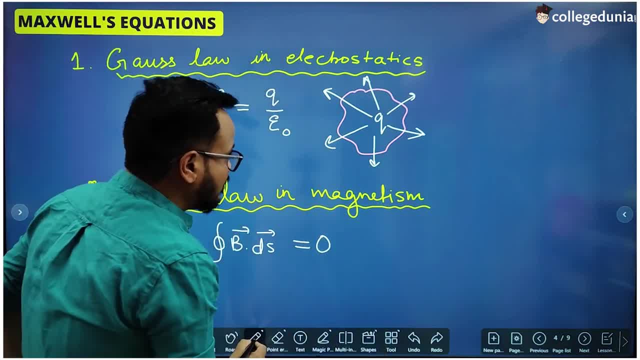 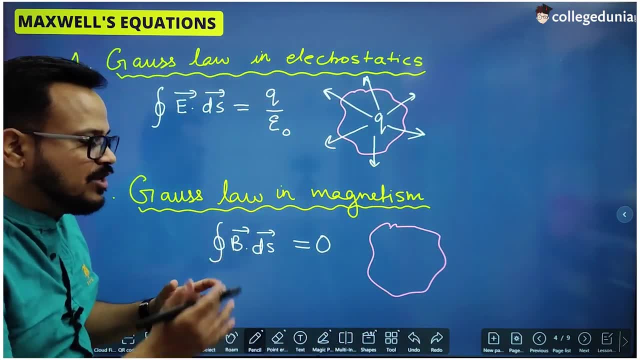 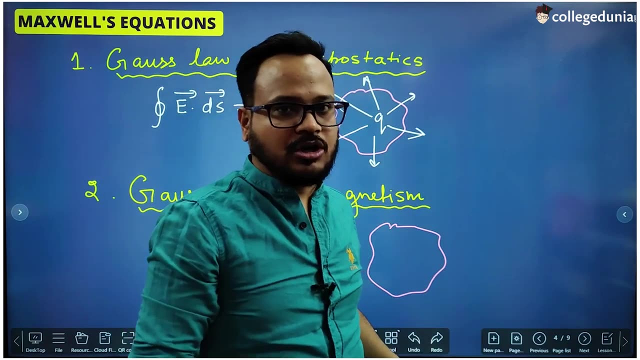 poles exist together in magnetism. so if there is a closed surface like this and this surface contains a source of magnetic field, then obviously both north and south poles are there. so the total number of magnetic field lines which are coming out of this surface due to the north 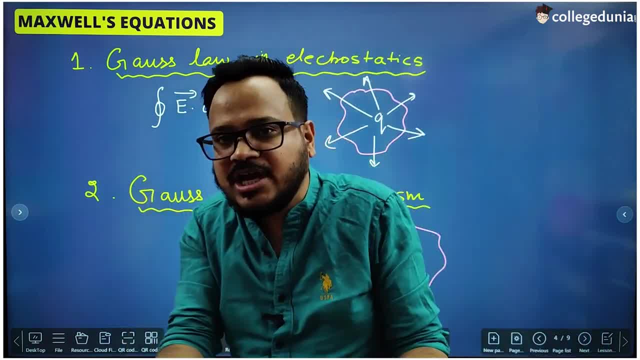 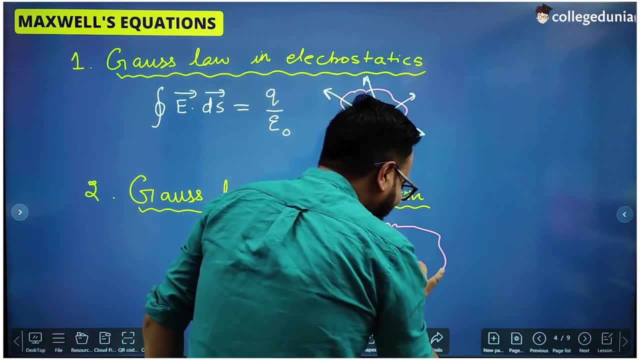 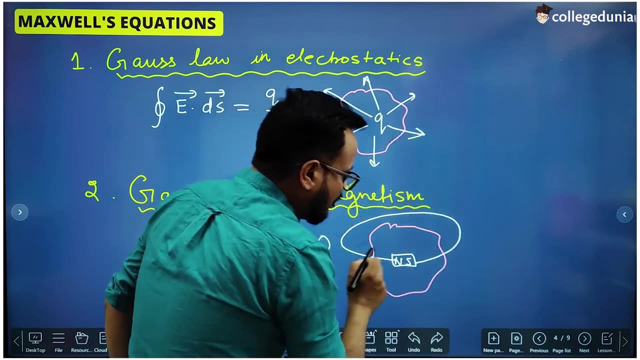 pole is equal to the total number of magnetic field lines which are going into the surface because of the south pole, so that net flux, not netflix, it is net flux. so if, suppose, a bar magnet is placed here, so magnetic field lines will emerge from north pole and they will 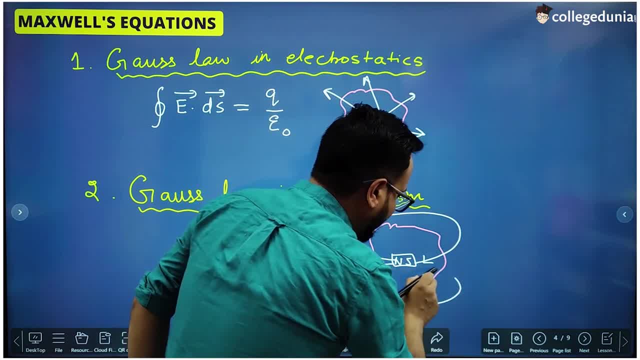 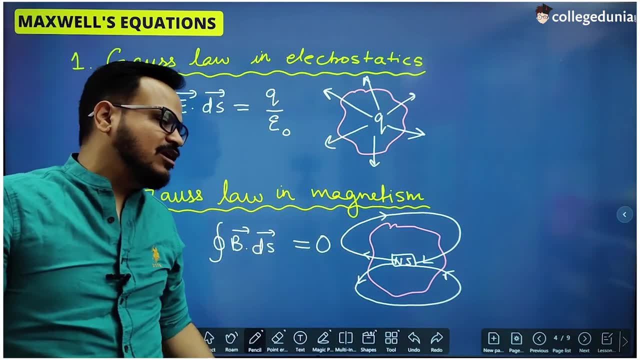 go through the closed surface by going into the closed surface. so if there is a source of magnetic field, go into the south pole and if this is the second magnetic field line which is going out of north pole and coming back into the south pole. so if we count each and every magnetic field line, we will. 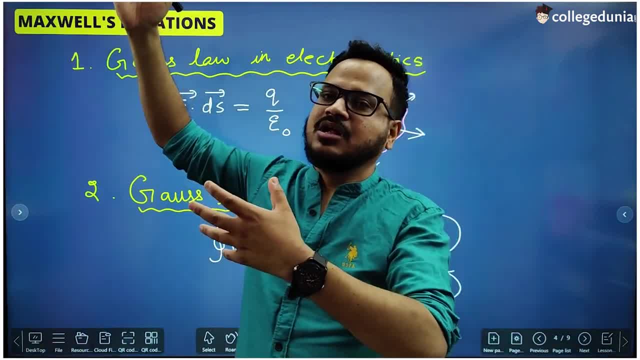 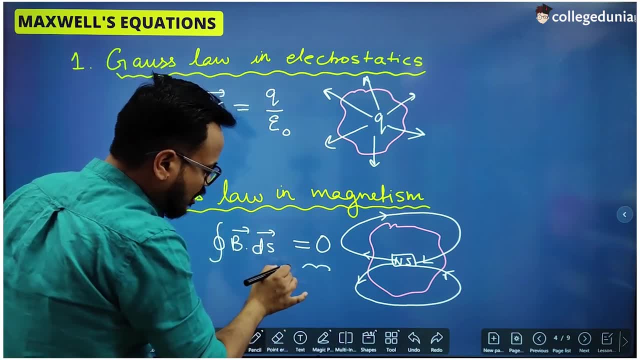 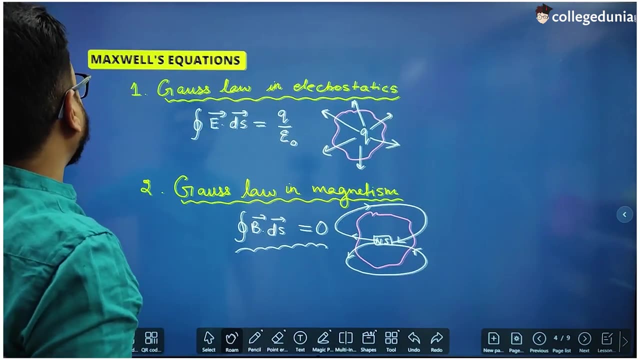 say that the total number of magnetic field lines which are leaving the surface is equal to the total magnetic field lines which are entering the surface. so the net magnetic flux through a closed surface is always zero. right, this was the second, or this is the second maxwell's equation. okay? 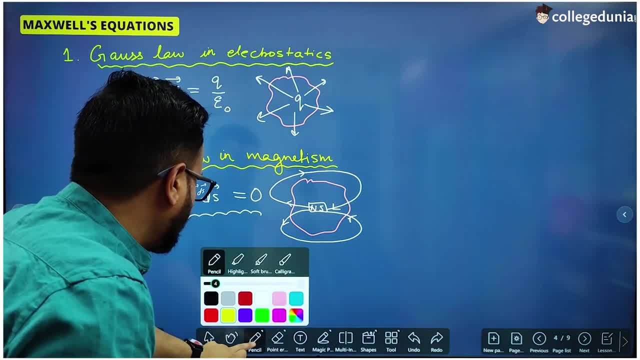 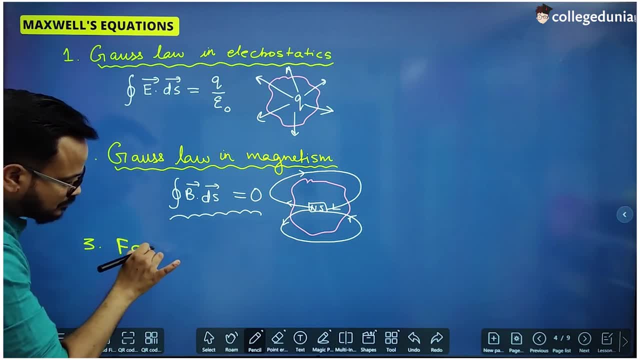 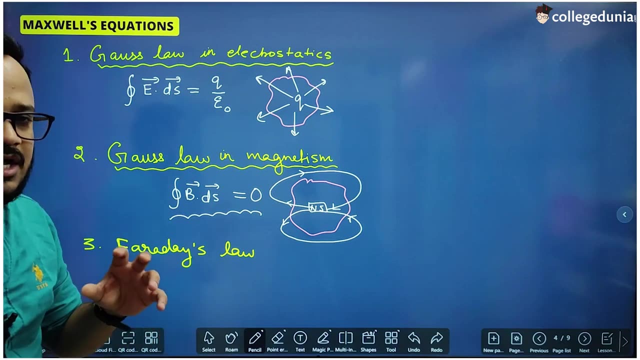 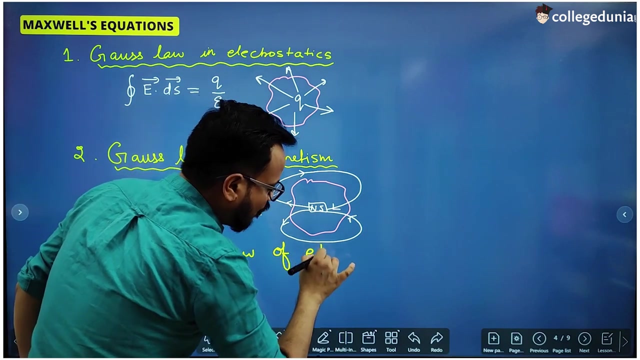 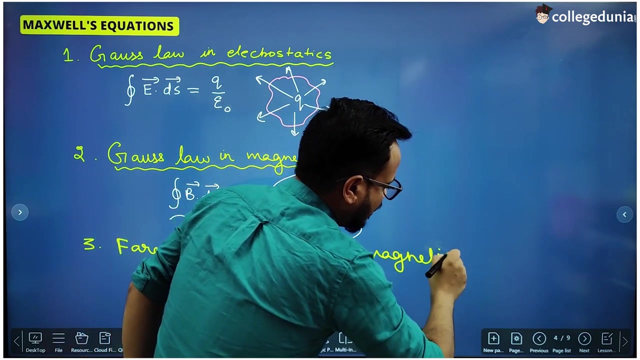 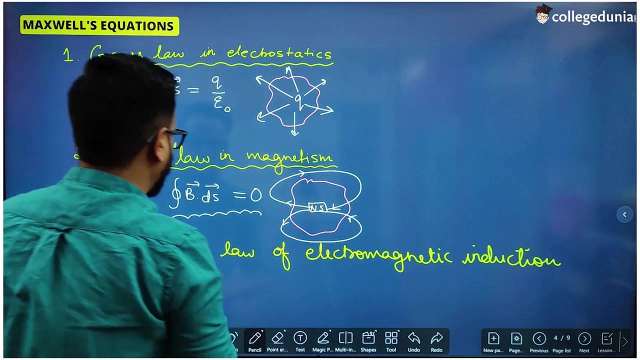 from the concepts of, from the topic of electromagnetic induction, maxwell picked faraday law. second law, first law of faraday does not contain any mathematical equation, so faraday's law's law, second law of electromagnetic induction, electromagnetic induction. this is your third maxwell equation, okay. 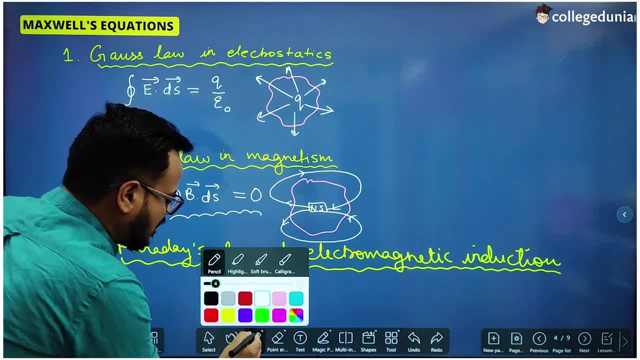 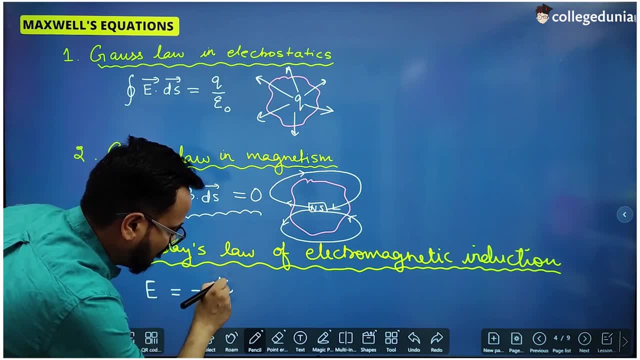 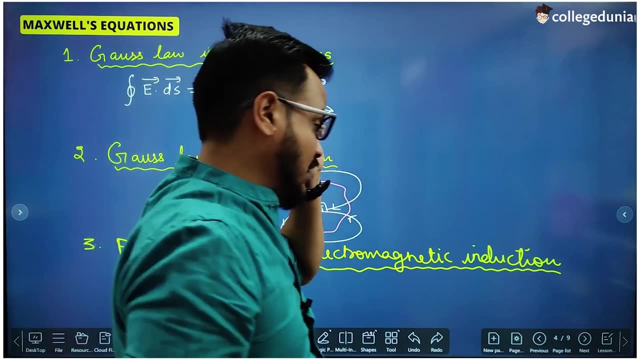 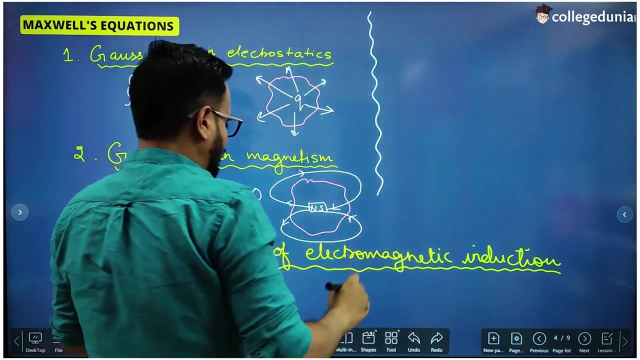 what is the equation in faraday's second law? it says that the emfe is is, is is the rate of change of magnetic flux. that is minus d phi by dt. right, this e is emf, not electric field. emf means the potential difference or the voltage, right? okay, we know that. what is magnetic flux? 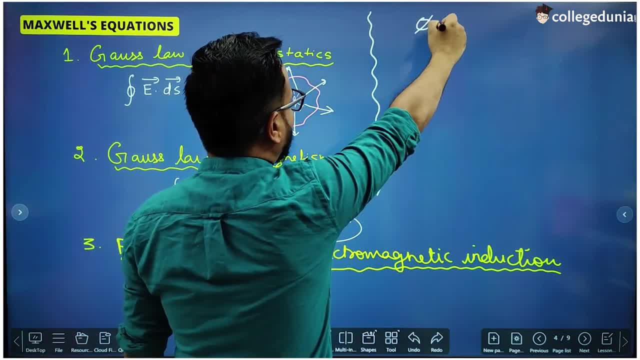 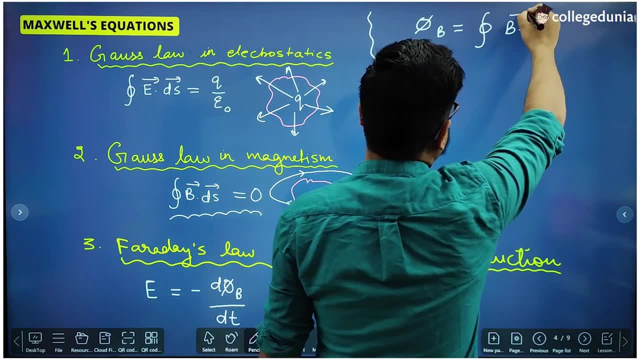 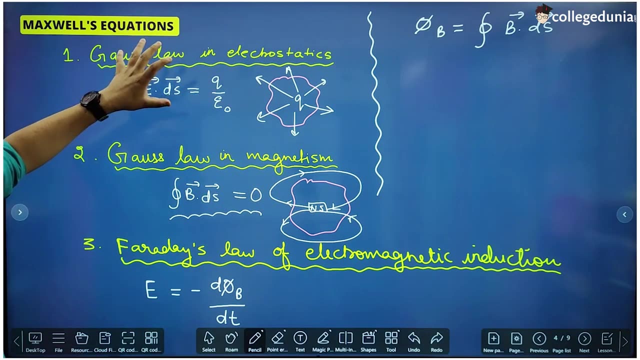 magnetic flux is simply b dot ds, so in place of phi b. if we write in class 12, we just have to remember these equations. we don't have to use these equations to solve any question. these equations are used in their respective chapters. but in electromagnetism 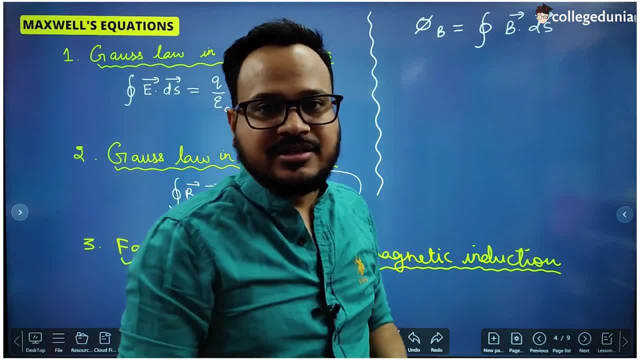 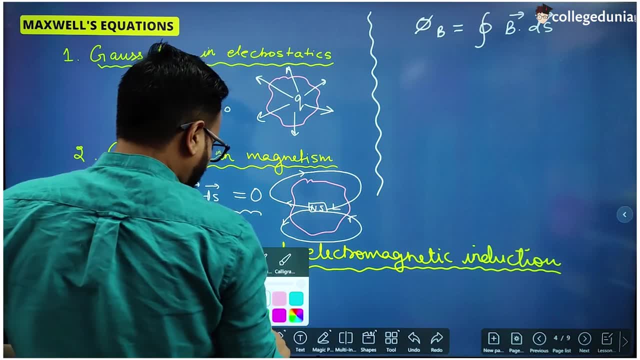 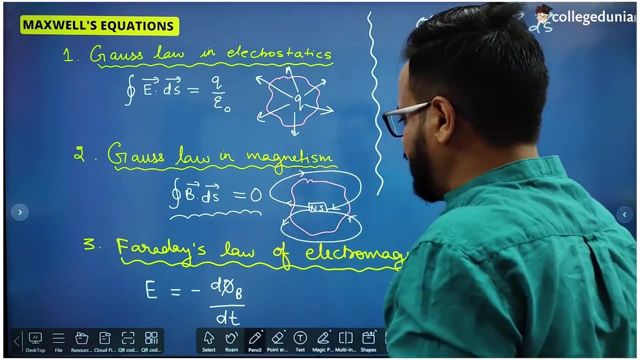 in in sorry electromagnetic waves chapter. these equations are used to explain the concepts of electromagnetic waves, so we just have to remember these equations, right? so phi b can be written as b, dot, dx, integral right, and we know that. electric field, or? or we should write it v. 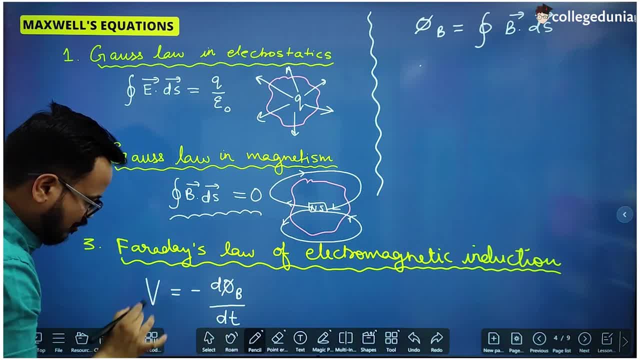 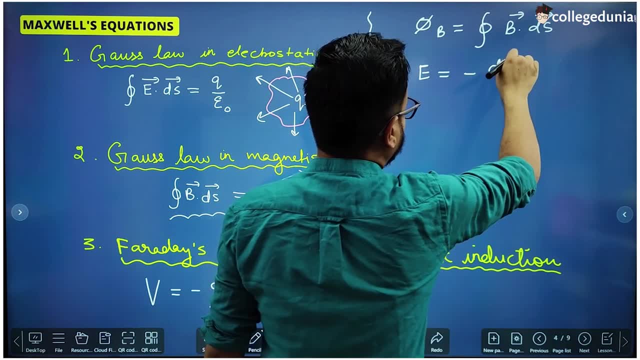 b, dot, dx, integral right. and we know that electric field or- or we should write it- v, Otherwise you will get confused between V and E. So this is the potential V right. And in electrostatics we have learned that E electric field is minus dV by dr, So we can write V as. 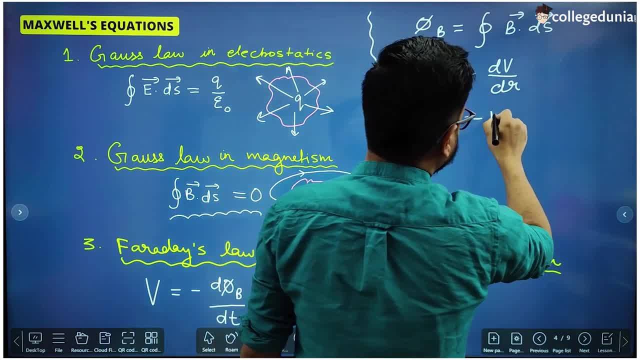 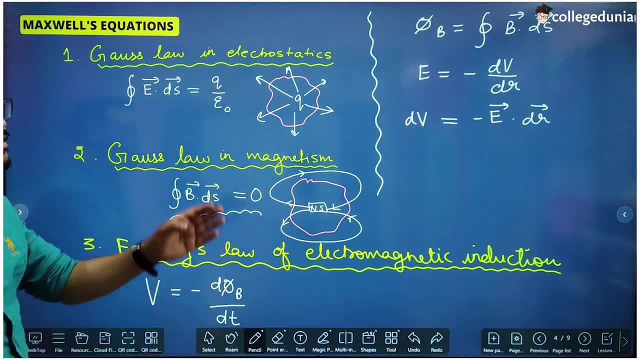 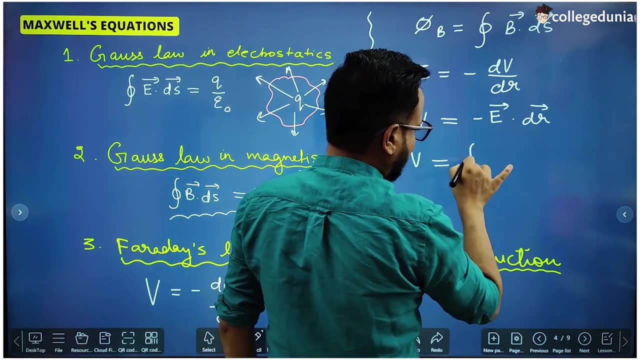 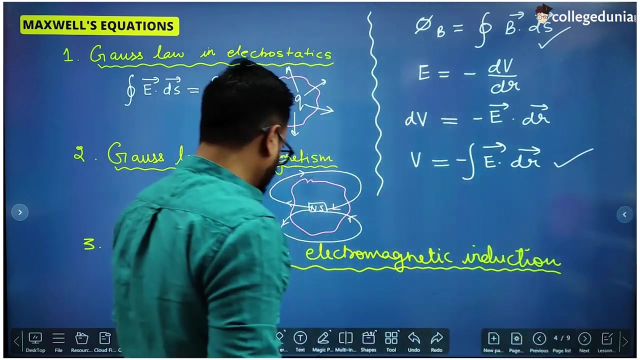 or dV as minus E dot dr. right, Because potential is scalar quantity and E and dr are vectors. Then obviously dV is the dot product of E and dr. So if you will integrate this, you are going to get V as this. It is the integral of E and dr. Now, if we put this and this in the 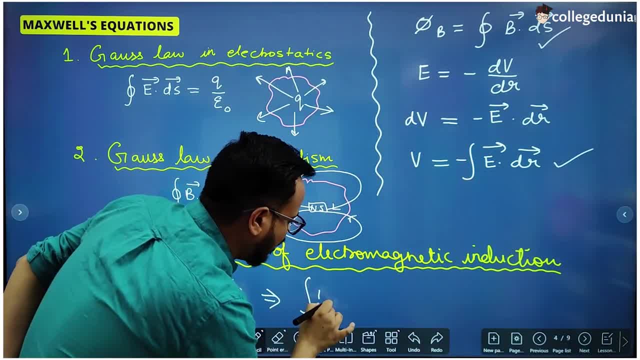 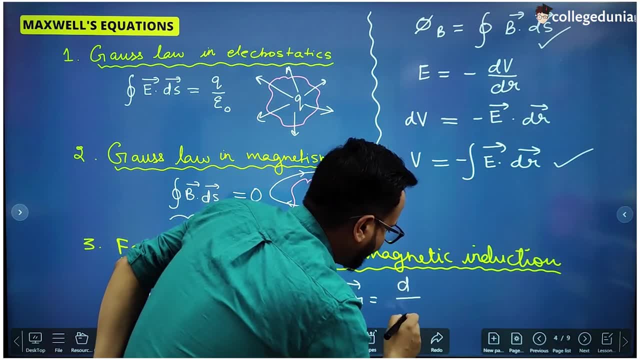 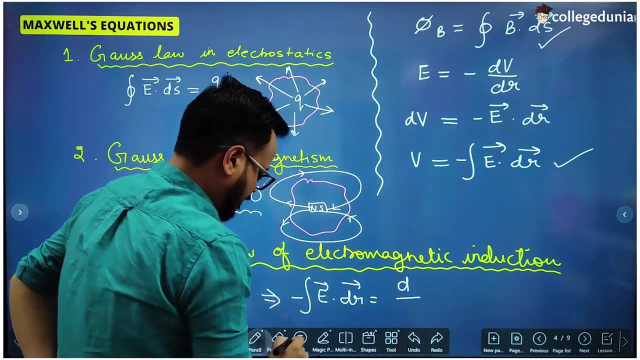 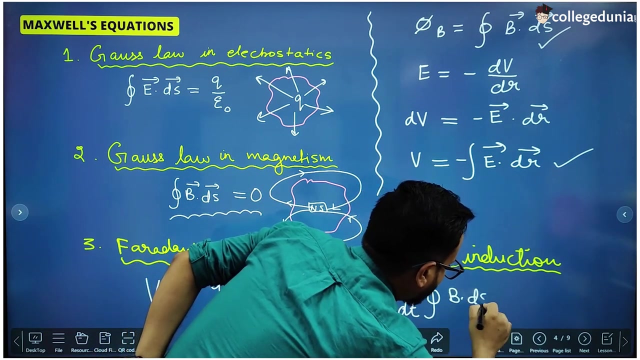 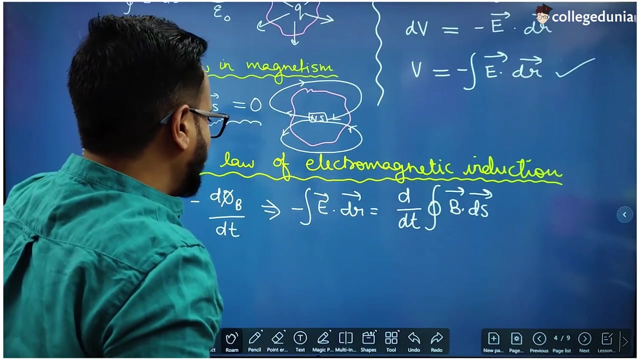 third equation. so this equation becomes the integral of negative of E. dot dr is equal to the derivative of with respect to time, sorry, the derivative of magnetic flux with respect to time, right? So this is Maxwell's third equation, right? And the fourth equation is the modified Maxwell. 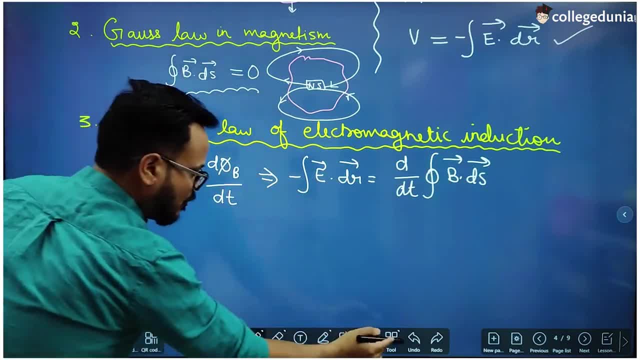 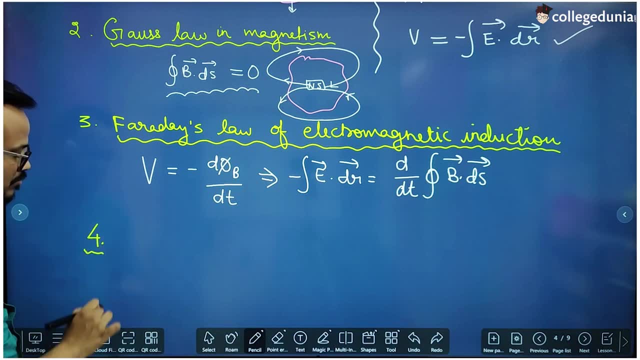 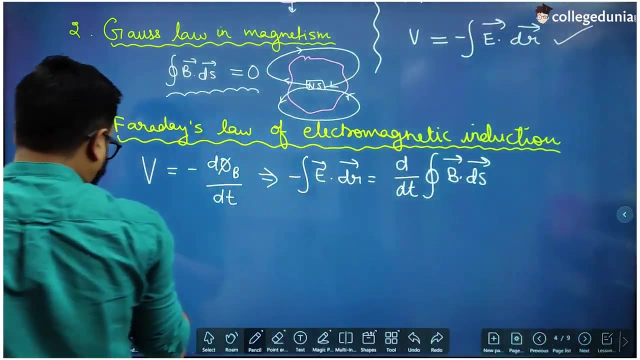 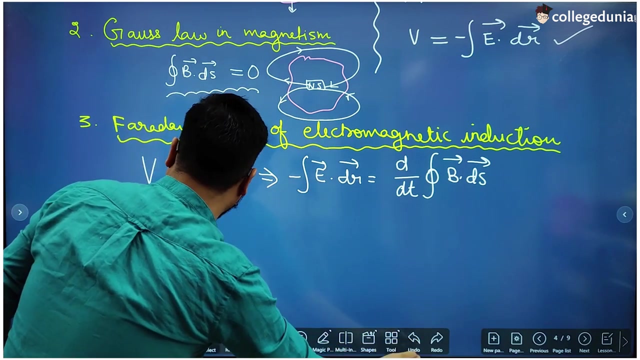 Ampere Circular Law. Fourth equation is the modified Maxwell Ampere Circular Law, Because modified the Ampere-Circular law and then that law becomes the modified Ampere-Maxwell-Circular law. So that is the fourth equation modified, or we can simply write: So if we include: 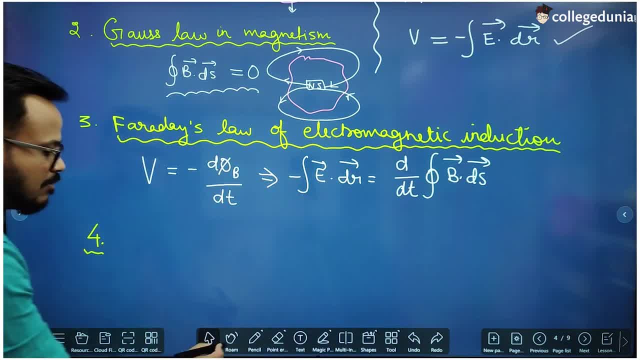 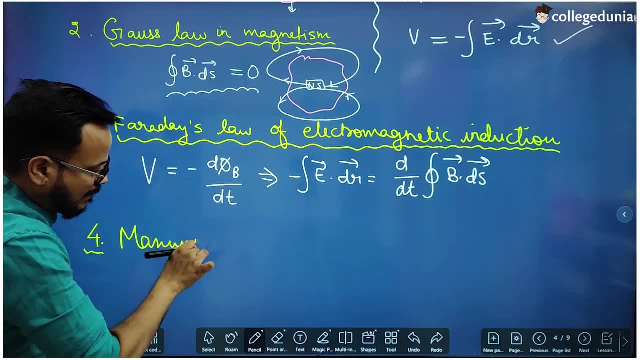 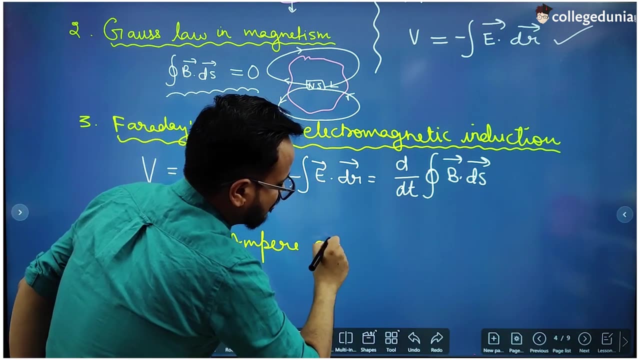 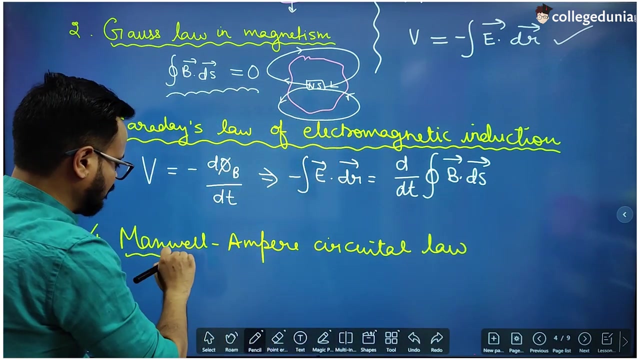 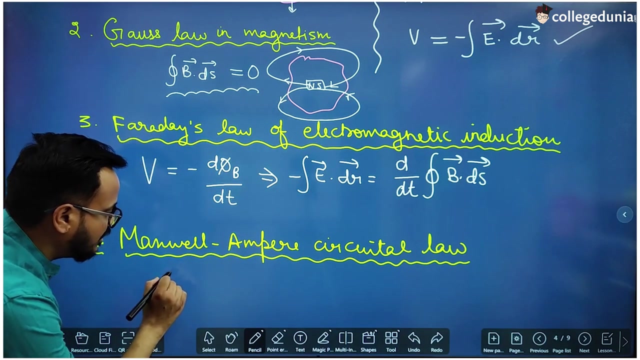 Maxwell's name and Ampere-Circular law. that means we are talking about the modified form of Ampere-Circular law, So it is called Maxwell-Ampere-Circular law. And what was that Maxwell-Ampere-Circular law, which says that